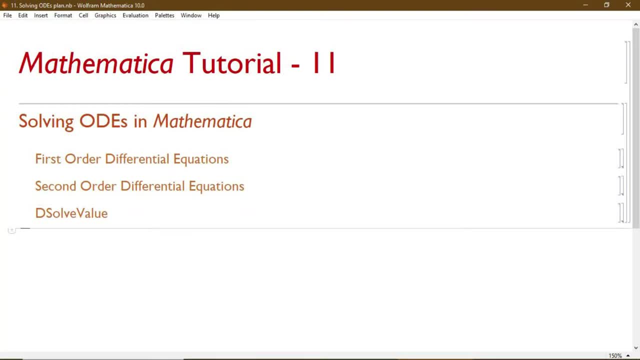 Hello everyone, welcome to 11th Mathematica tutorial and in this video I am going to discuss how to solve differential equation first order and second order in Mathematica. So let's start the video. Let's start with this simple example. This is a differential equation: dy dx is equal to. 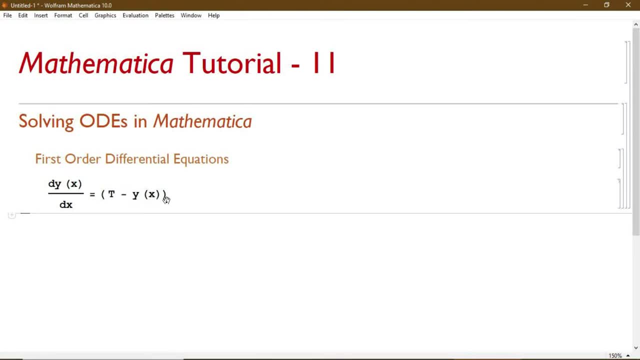 t minus yx, where t is some constant or some parameter. So to solve this differential equation in Mathematica we have to use this function, dissolve. and the syntax for this function looks like this: In the first argument you have to specify the equation that you want to solve. 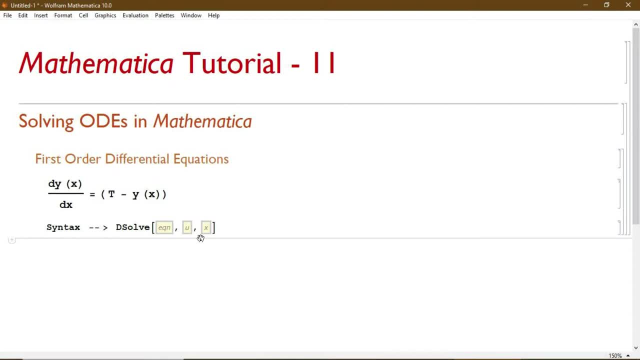 and in the next two argument you have to specify the variable and the parameter. Now you have to write this differential equation in Mathematica language. So any derivative in Mathematica you can write it like this: y prime x, that is derivative of y with respect to x, obviously, where y is a function of x. Now if you have a double derivative, then 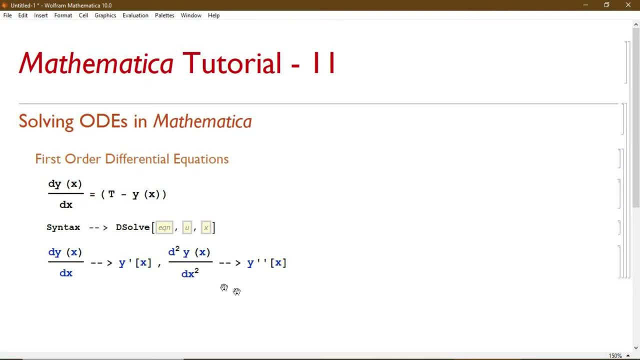 you can write it like this: dy dx square, which you can write by using double prime. So if you want to have higher order, all you will have to specify the order of differentiation. Let us see now what you can do If you want to have more order even without raising the 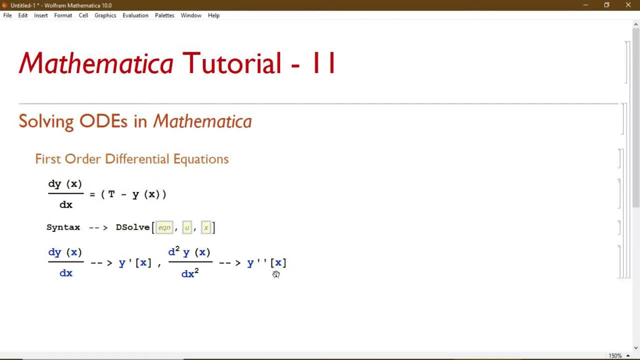 parameters. if you just want to make the reason of any attrition, you will have to use the differential equation. and to solve the differential equation, you we have to insert new variable term like: and remember, you will have the element ofThrough horses and, as you can see, I want to have 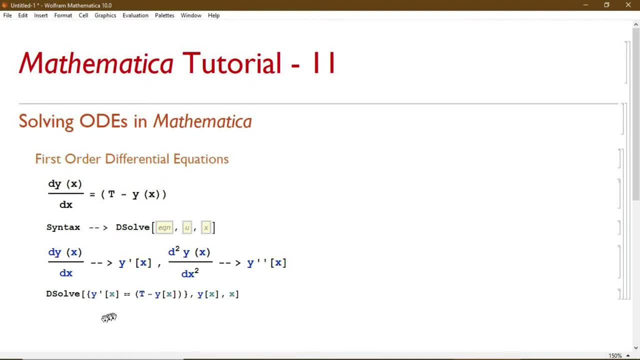 different limit as a general term. So let's solve this equation. So when you know that the and I have the learnt to match shape on first and second», dy, dx, and you have to put double equal, then write t minus yx, and as y's are the function of x, then 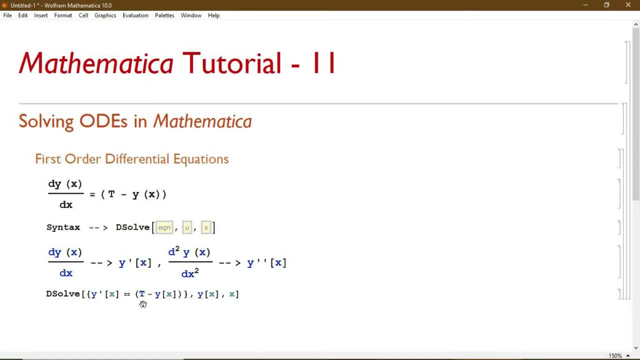 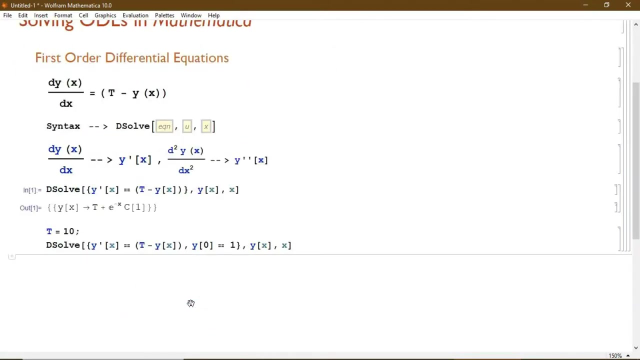 so you have to write x in the square brackets and i put this differential equation in a curly braces. so next i specify the variable y and i specify the parameter on which the y depends. now, if you evaluate this cell, then Mathematica will give you the answer. now you can also specify the. 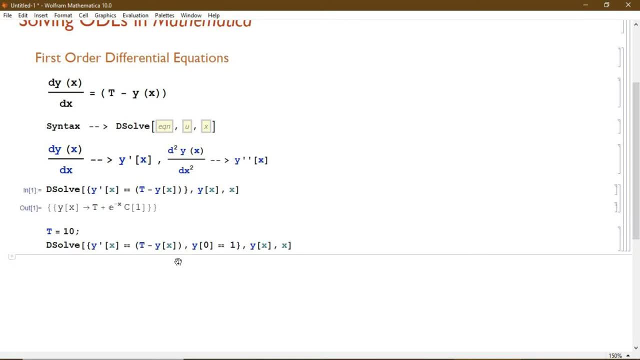 initial value or the boundary conditions, or you can also specify the value of the parameters. as you can see, in this solution there is a constant c1. so, as it is a first order differential equation, obviously there is one, one constant only now, to evaluate this constant, you have to specify one initial condition. so i: 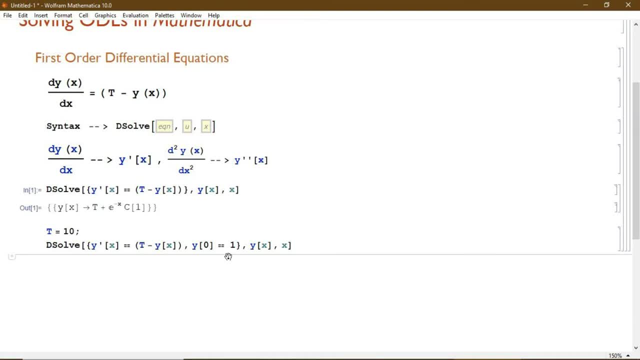 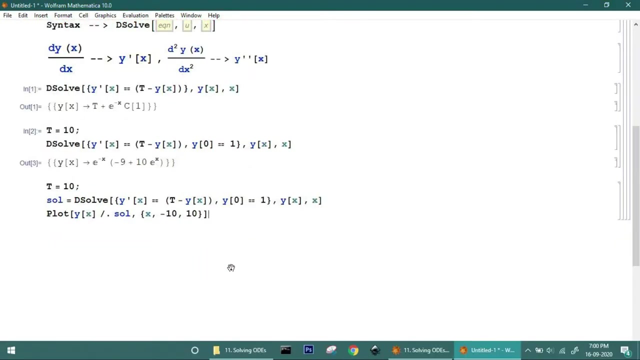 specify at: x equals to 0, y is equals to 1.. so now, if you evaluate this, this will give your answer. so this is the answer of this differential equation, with this parameter t assigned to value 10 and with this initial condition. now the next thing: yeah, say, if you want to plot the 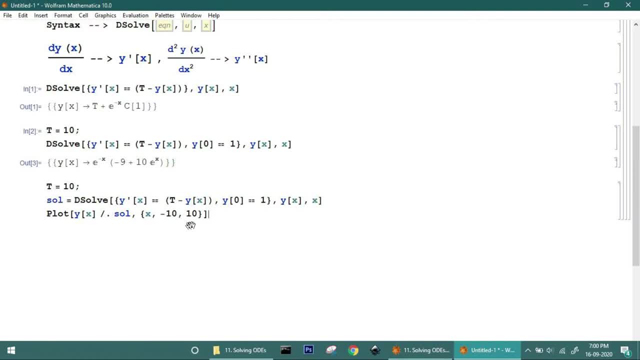 solution with x ranging from minus 10 to 10. then you can write it like this: plot yx- slash dot. this is the replacement operator and i want to plot yx from the solution. okay, so i write sol equals to dissolve and this thing, and now i want to plot this yx. that is the solution within the range minus 10 to 10. 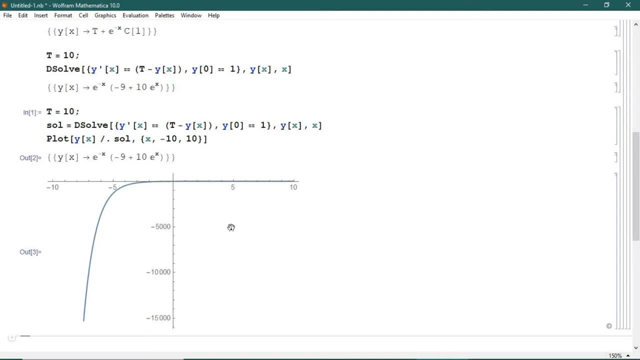 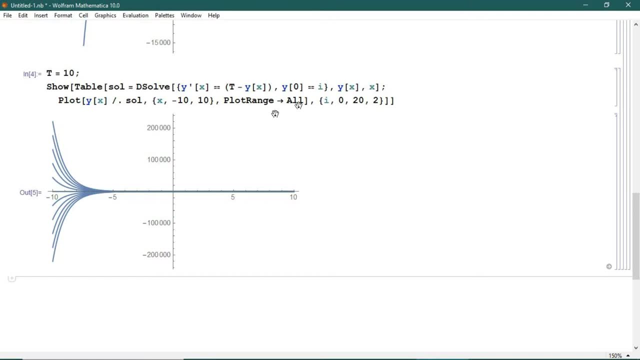 so now this will look like this. now say, you want to solve this differential equation for various initial conditions. so, as you can see here, i put y, 0 equals to i. now i make a table where i varies from 0 to 20 within a step 2 and i plot y and i, uh, so all of the graphs in the same plot. that's why. 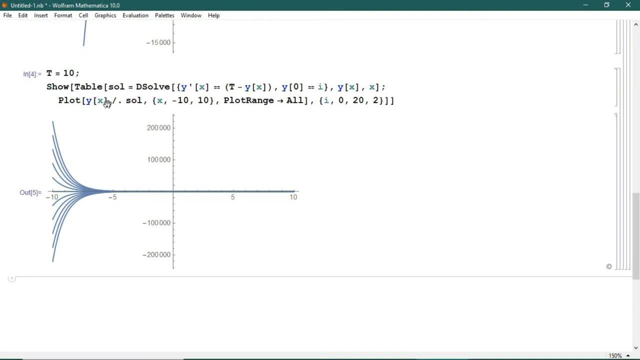 i use this uh so function. i already had discussed about all of these functions in my previous videos. so this is the family of solutions for different initial conditions. now you can also find the solution for different values of this parameter t. so now, as you here, as you can see, uh, i write this, i or this, i assign. 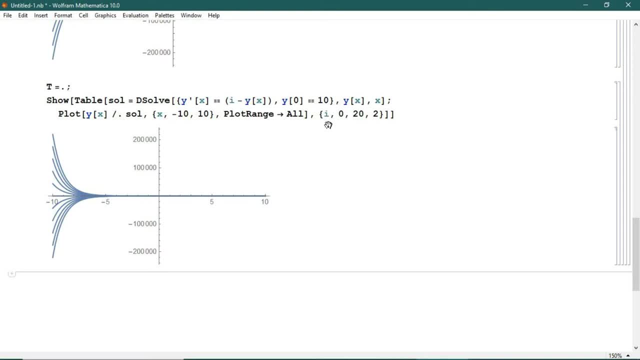 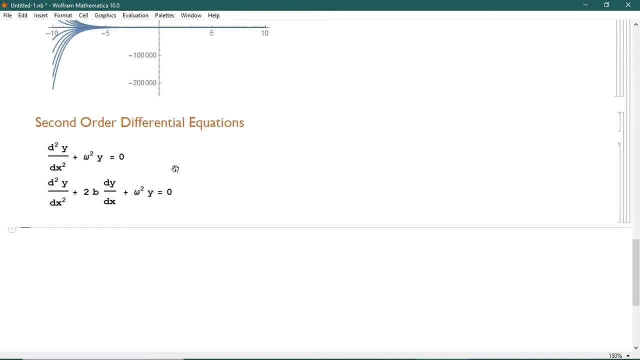 this variable i instead of t, and i changes uh the value of i from 0 to 20 within a step of 2, and this is the family of solutions, uh, for these different values of t. now let's come to the second order differential equation. so 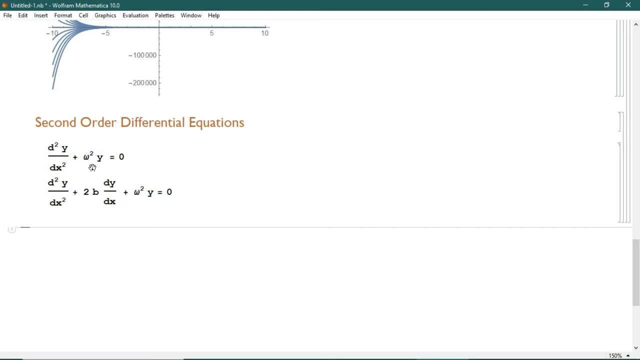 second order differential equations. one is corresponds to undamped harmonic motion and the other is damped harmonic oscillator. so to solve this i use this dissolve function again and i write this d2y dx square as y double prime x equals to minus omega square yx. you can also write y double prime x plus omega square yx equals to zero. both are same. 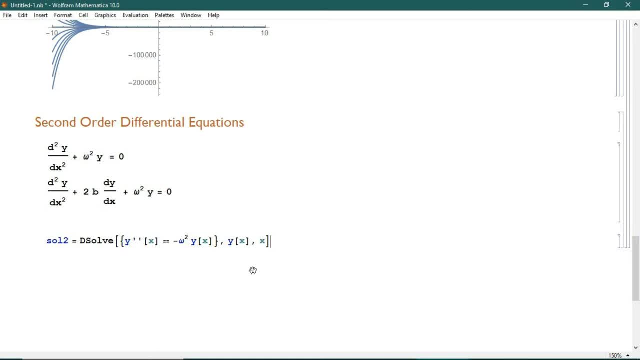 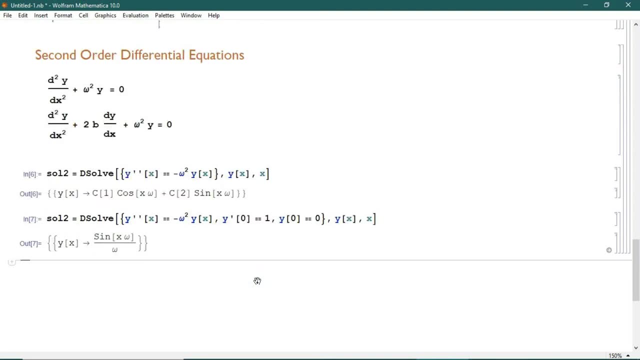 okay, then i specify these two arguments. and now, if if you evaluate this cell, it will give your final answer again- you can specify some initials condition to evaluate this constant c1 and c2 now, as it is a second order differential equation, so you have to specify two initial conditions. so 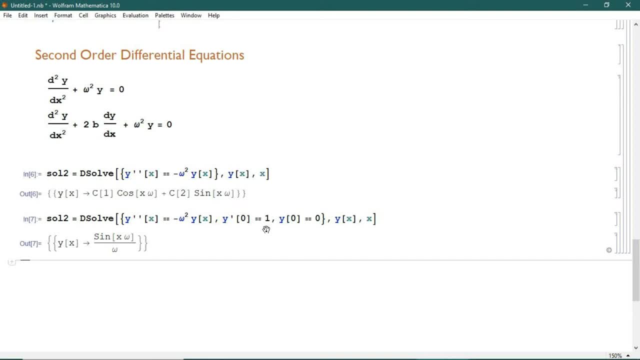 i specify: y, prime, which is the velocity term, equals to one and y, which is the initial position of the particle, say, which is zero. okay, so this is my solution. now, if you want to extract this solution from this thing, then you can use this command or you can construct a function. 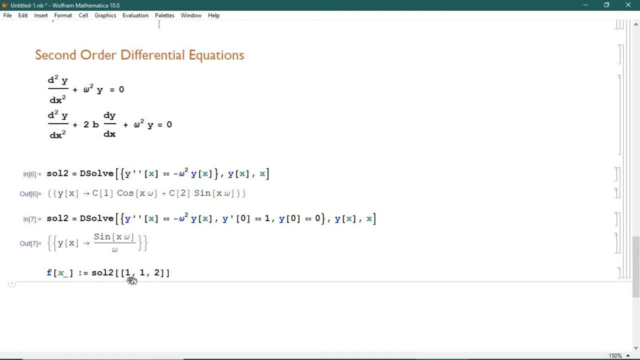 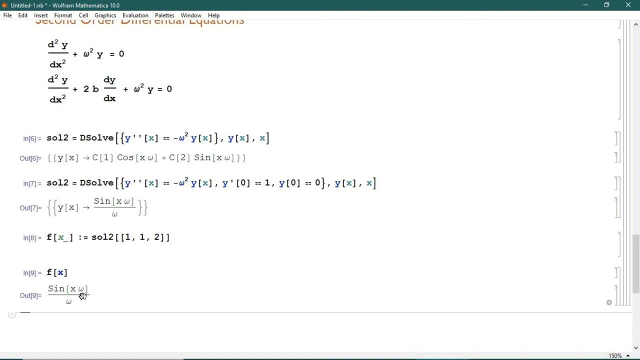 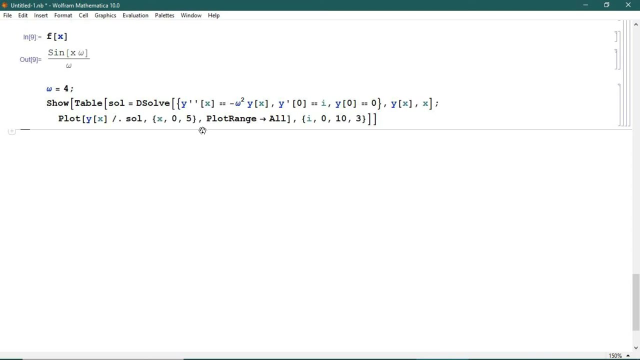 like this. so 112 means first row, first column, and the second element. so fx is equals to sine omega, x by omega, which is this solution. so now if you want to plot it, say for various initial values of y prime, then you can do it as. sorry before. so I construct a table from zero to. 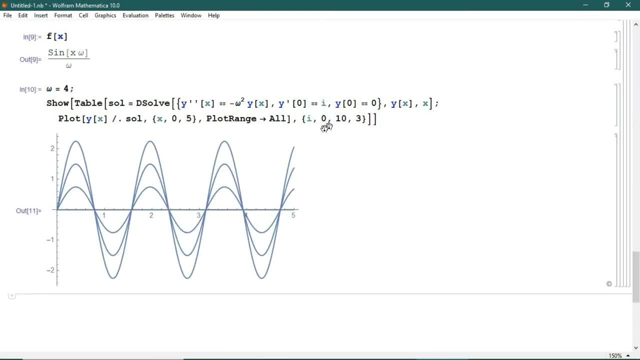 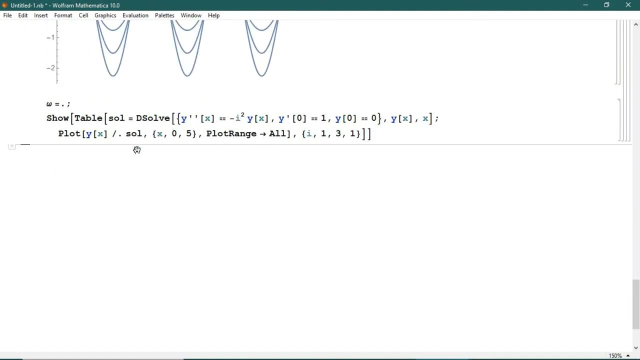 to 10 within a step of 3, and I specify this variable, or this initial condition, with i, and if you evaluate the cell, it will give this family of solutions for omega equals to 4.. So now, if you want to vary this frequency, then you can also do it like this, and if you plot it, 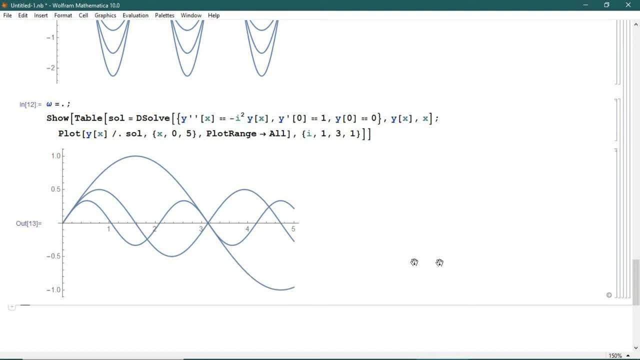 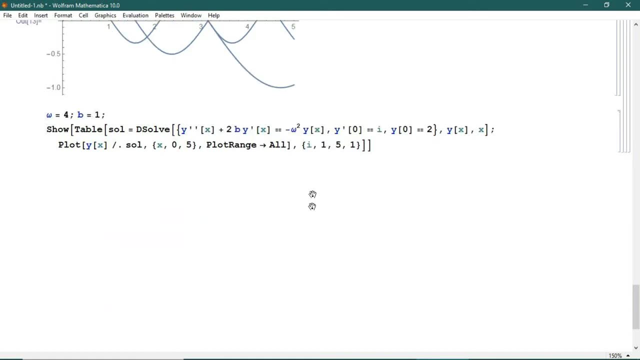 it will show such curves. So here I vary omega from 1 to 3 within a step of 1.. Now let's solve this equation for damped harmonic oscillator. So, as you can see, here is a new parameter or new term, to be y, prime x, or to be dy, dx. So I specify the value of b and I. 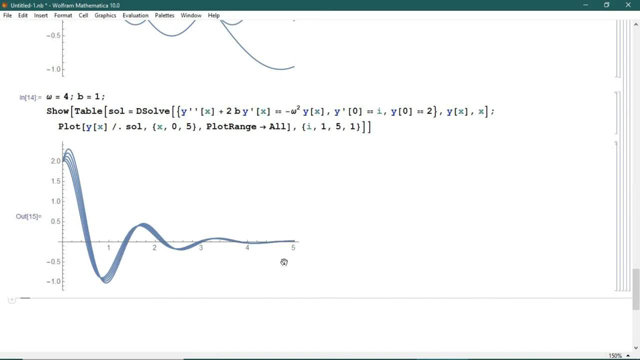 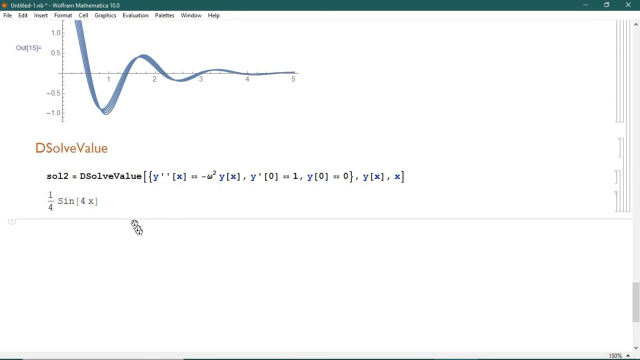 plot it and, as you can see, it shows the damped motion, and this is how you can solve differential equations in Mathematica and plot it, or you can find the family of solutions like this, and whatever you want to do. Another thing is you can use this function, dsalveValue, to directly. 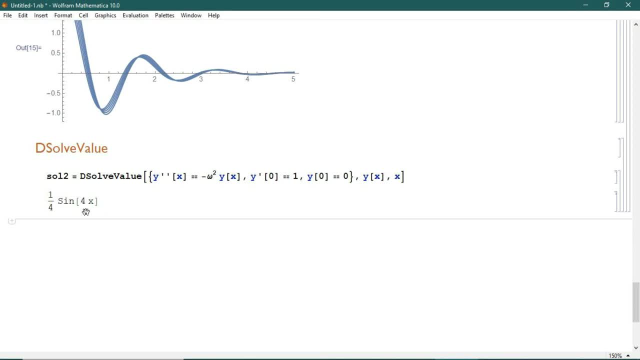 express the Bernieised equation with special olmaz. So, for example, you can plain delete, count the solutions from this equation. so, as you can see, and this gives you the direct solutions, which is 1 by 4 sine 4 X. actually, what happens here is that I 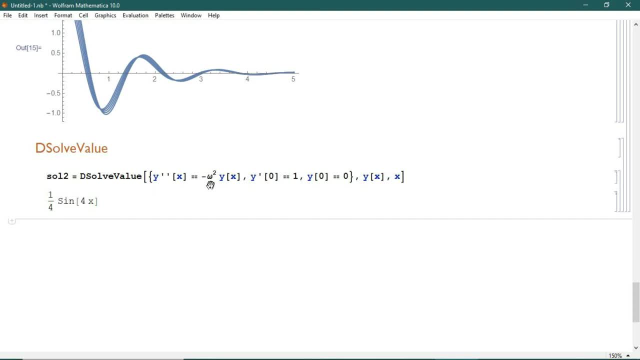 previously assigned. the value for Omega equals to 4, so it takes this value, so that's why it's it keeps the solution like this. so see you in the next video. and in the next video you, I, will discuss how to solve couple differential equations in Mathematica.